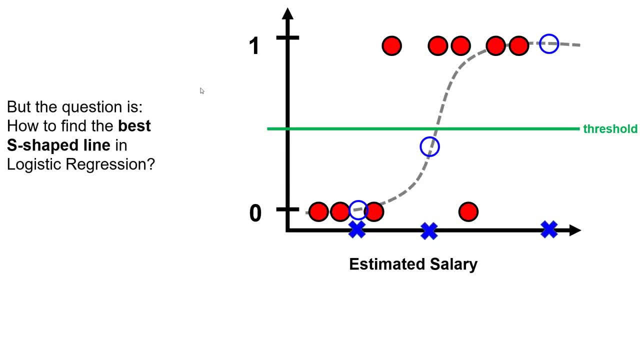 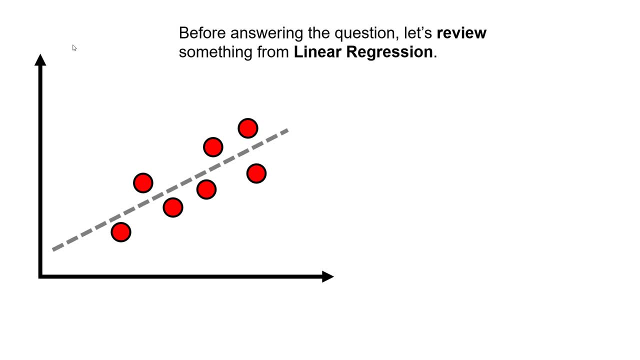 can have different kinds of variables as well, But the question is how to find the best S-shaped line in logistic regression. Before answering the question, let's review something from linear regression. In linear regression we try to fit a straight line. 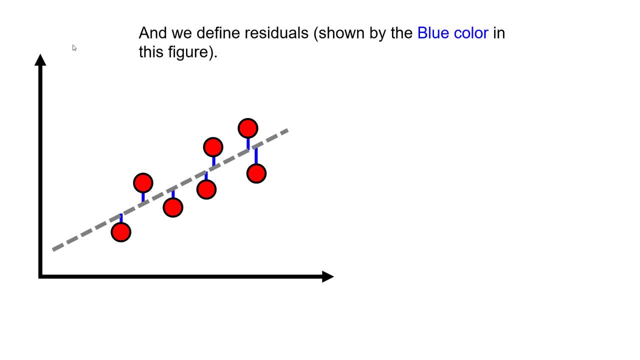 And we define residuals shown by the blue color in this figure And we try to find the best line that minimizes these residuals. So this is how to find the best line in linear regression, But in logistic regression we don't have the same concept. 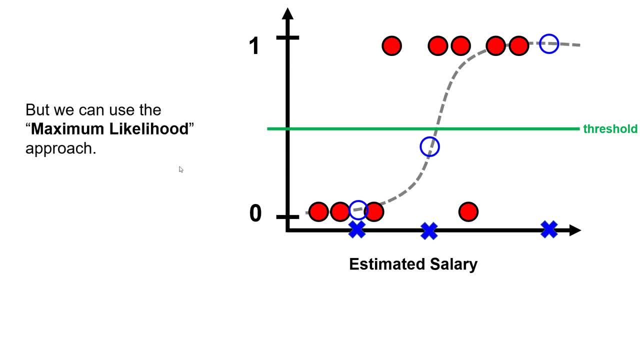 of a residual, But we can use the maximum likelihood approach. So maximum likelihood is a topic of another video. But in a nutshell, first you should pick an S-shaped line like the one you're seeing in this slide. Then you should calculate the likelihood or probability of seeing each data given this line. 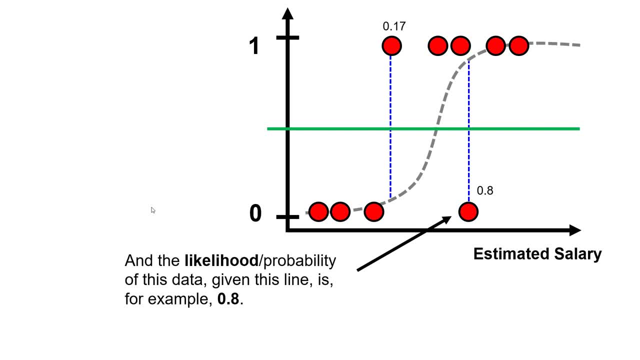 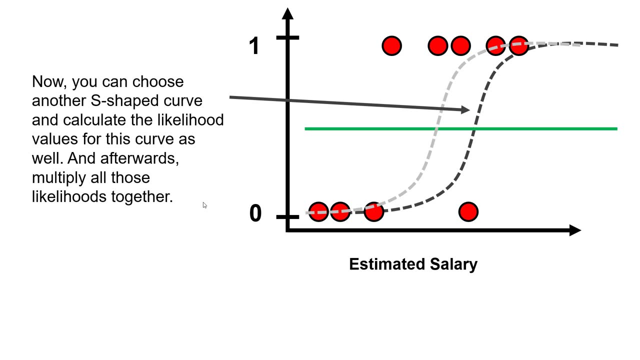 this data, given this line is, for example, 0.8.. And you can calculate other likelihoods or probabilities given this line, And then you should multiply all these numbers And if you do so, this would be the result. Now you can choose another S-shaped curve and calculate the. 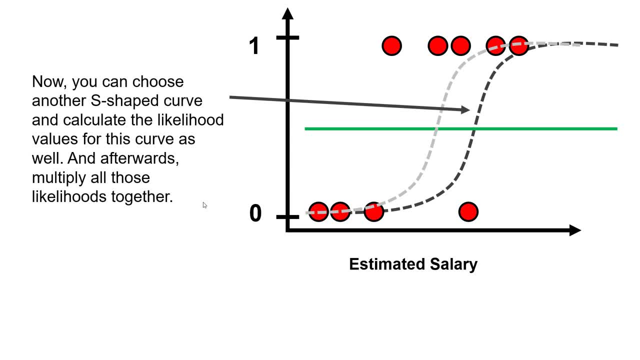 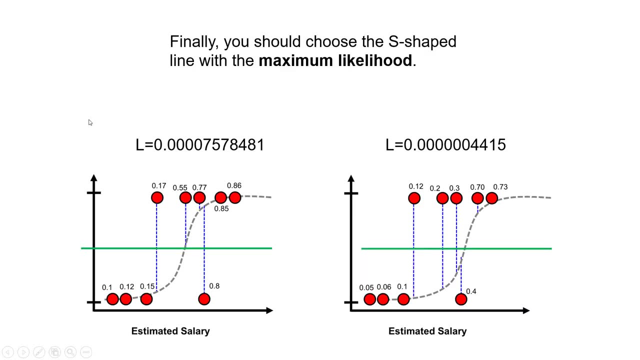 likelihood values for this curve as well, And afterwards, multiply all these likelihoods together, And if you do so, this would be the result. You can try other S-shaped curves as well, But let's keep it simple and work with these two curves. Finally, you should choose the S-shaped. 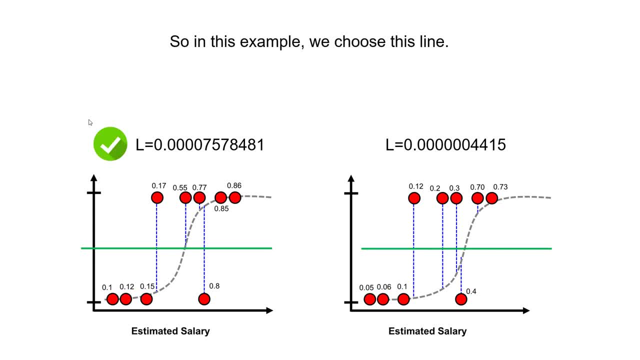 line with the maximum likelihood. So in this example we choose this line. Terminology alert: In this context you should use the term likelihood instead of probability, But in previous slides I used the term probability as well. for those people not familiar, 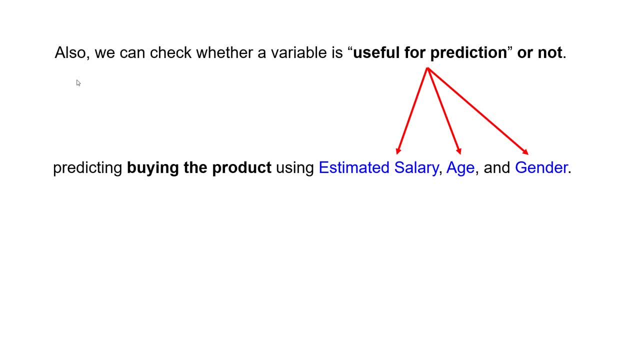 with the topic. Also, we can check whether a variable is useful for prediction or not. Using a statistical test called Wald's test, we can test whether the effect of a variable on the prediction is significantly different from zero or not. If the effect of a variable